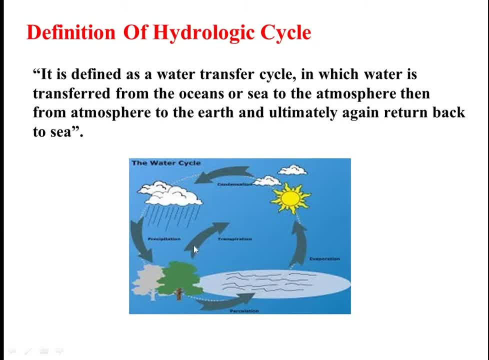 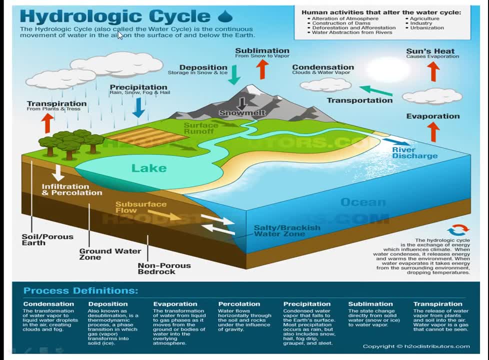 Below mentioned figure shows the how hydrologic cycle takes place. Hydrologic cycle, also called water cycle, is the continuous movement of water in the air, on the surface of and below the earth. This cycle is exchange of energy, which influences climate. When water condenses, it releases energy and warms the environment. 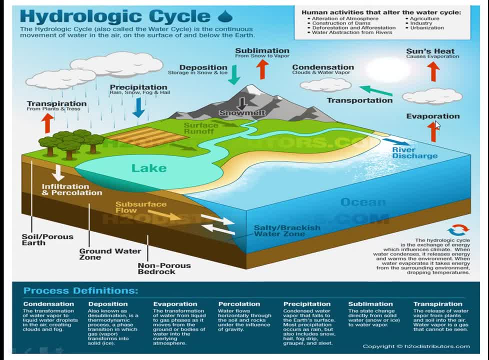 When the water evaporates, it takes energy from the surrounding environment, dropping temperature. Hydrologic cycle: action in field. Hydrologic cycle is a cycle which describes the storage and movement of water between the biosphere, atmosphere, lithosphere and hydrosphere. 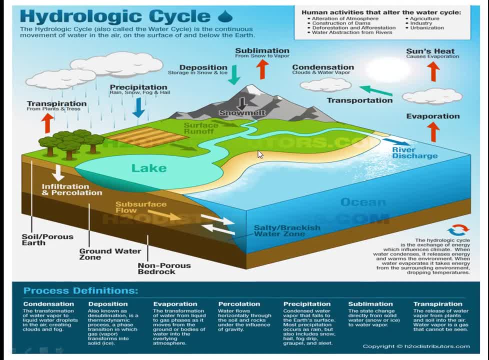 Water on our planet can be stored in major reservoirs: atmosphere, oceans, lakes, rivers, soils, glaciers, snow fields and groundwater. Water moves from one reservoir to another by way of process like evaporation, condensation, precipitation, transpiration. 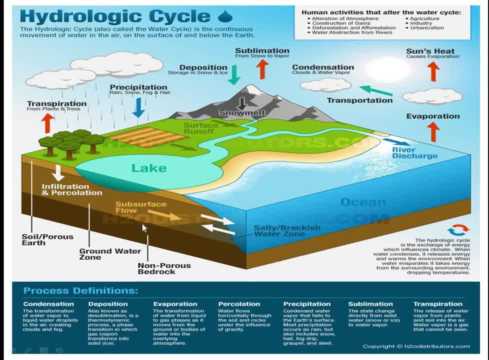 melting and groundwater flow. The oceans supply most of the evaporation water found in the atmosphere. The resulting imbalance between rates of evaporation and precipitation over land and oceans is corrected by runoff and groundwater flow to the ocean. Evaporation takes place from the surface of ponds, lakes, reservoirs, oceans surface, etc. 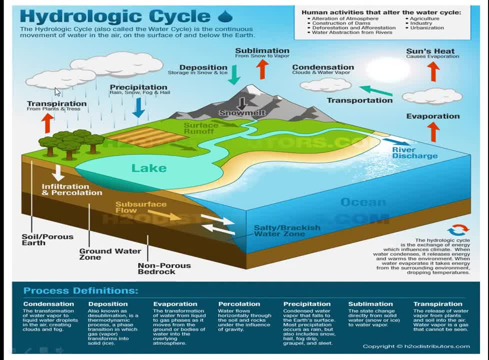 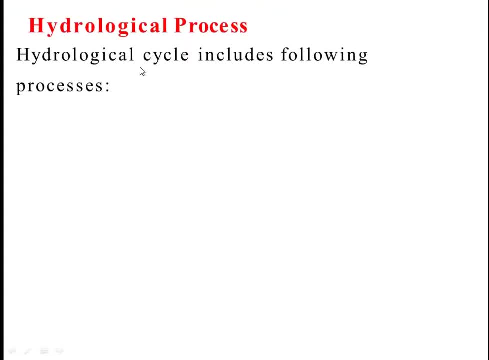 and transpiration from surface vegetation and other types of vegetation, as shown in figure. Coming to the hydrological process, Hydrological cycle includes following processes: First one is the evaporation. Second one is the condensation. Third one is the precipitation. Fourth one is the intercipation. Fifth is the infiltration. Sixth is the percolation. 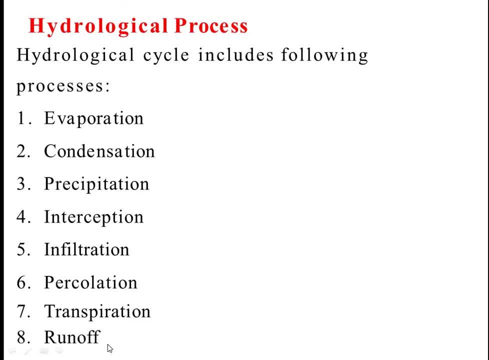 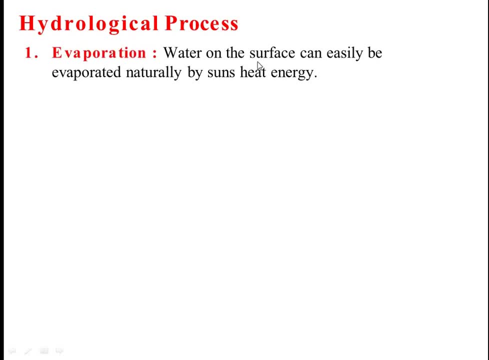 and seventh is the transpiration and last is the runoff. Discuss hydrological process one by one. First one is the evaporation. Water on the surface can be easily evaporated naturally by sun heat. energy as shown in figure Occurs when water changes from liquid state to gaseous state. 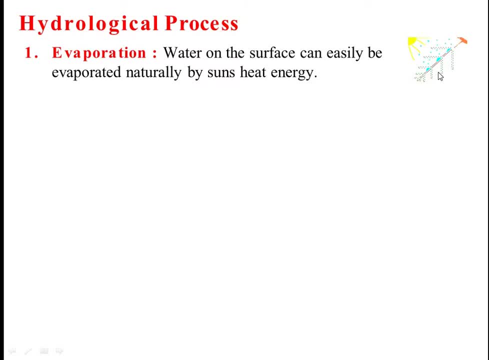 It occurs on water surface, like lakes, seas, etc. Evaporated moisture is lifted into atmosphere, but some vapor always exist in the atmosphere. Second one is the condensation. Condensation is processed, By which water vapor changes into water. As shown in figure, Water vapor condenses to form. 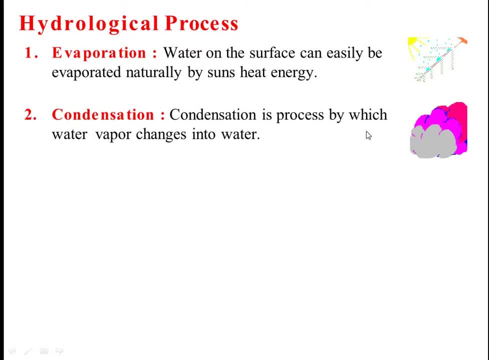 dew, fog or clouds. Condensation takes place due to cooling of air, That is, water converts into cloud form. Precipitation: It is the process that occurs when water particles fall from the atmosphere and reach the ground. Precipited water may fall into water bodies or on a land. 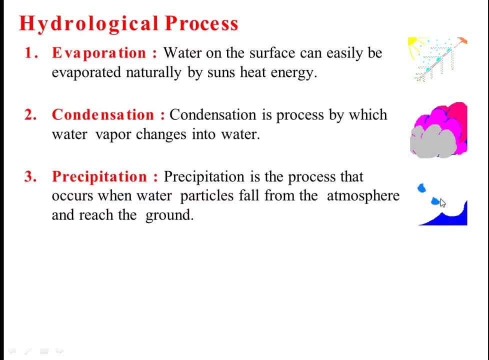 It can be a process of condensation. It can be a process of condensation, It can be a process of evaporation, It can go to streams or penetrate into the soil. Then intercipation is the process of interrupting the movement of water in the chain of transportation events: leading streams When rain. 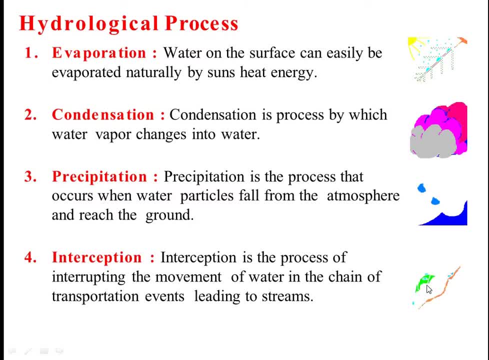 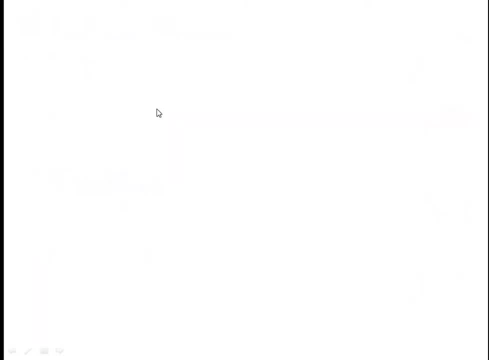 first begins, water striking the living and other materials spread over the surface or collects at points of edges, As shown in figure. Continuing with that, next one is the infiltration. Infiltration is the physical process involving movement of water through the boundary area, where 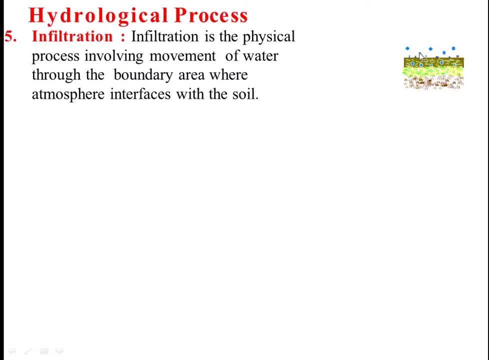 atmosphere interfaces with the soil. Infiltrated water and water stored in the soil can become subsurface runoff. Then percolation is the movement of water through the soil due to gravity and by capillary forces. All ground water originates as subsurface runoff. Then transpiration is the 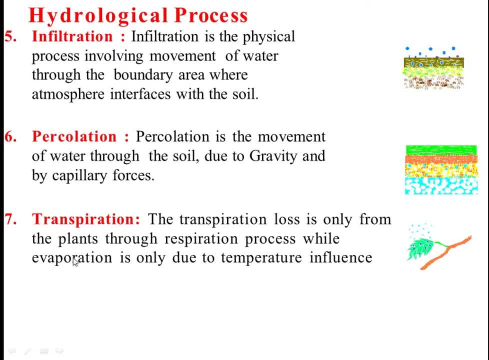 rapid acho mortis, where the decrease of water byety going through the soil with faster contraction helps if the spread of water GHmm factor changes. Next is respiration. The transpiration loss is only from the plants through respiration process, while evaporation is. 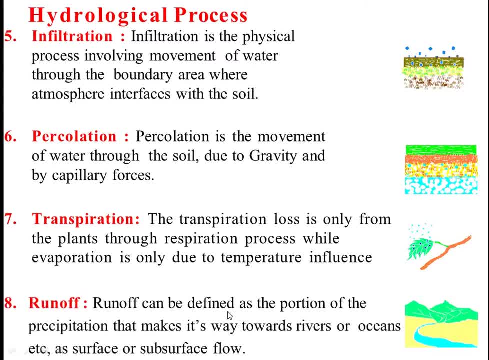 only due to temperature influence. Only small portion of water is retained by plants. Water inside plants is transferred to the atmosphere as water vapour, Then last one is the runoff, etc. as surface or sub-surface flow. It generally consists of flow that is unaffected by artificial. 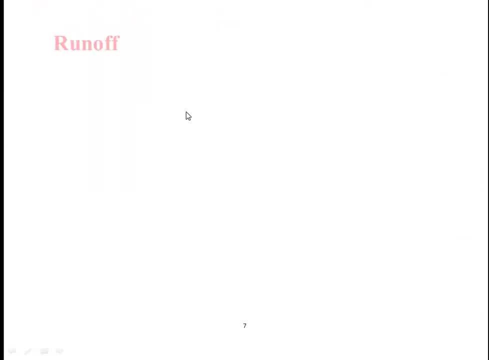 diversion or storages. A portion of precipitated water is intercipated by vegetation, building, ground surface etc. known as intercipation. The rest of water goes to the surface stream as surface runoff. Hydrologic balance equation is P equal to R plus E, where 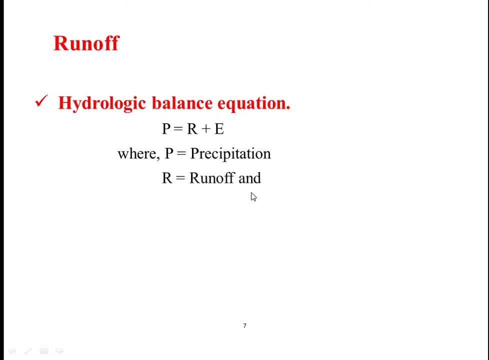 P stands for precipitation, R stands for runoff and E stands for evapotranspiration. Coming to the types of runoff, There are three types of runoff. First one is the surface runoff. second one is the sub-surface runoff, or interflow runoff. then third one is the base flow, or the 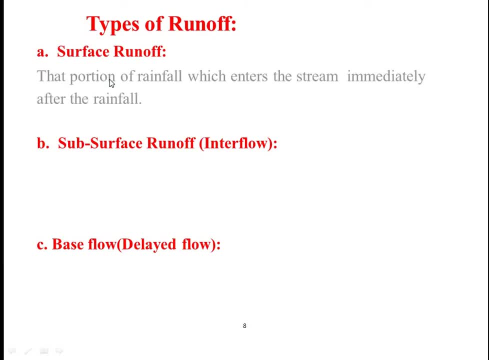 delayed flow. In surface runoff, it is that portion of rainfall which enters the stream immediately after the runoff. the rainfall, It occurs when all losses are satisfied and if rain is still continued with the rate of rainfall, that is, intensity greater than the infiltration rate. Then second one is: 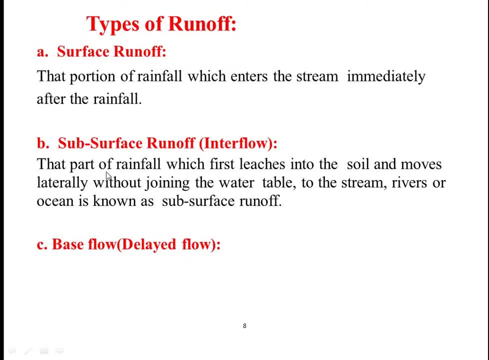 the subsurface runoff or interflow, That part of rainfall which first leaches into the soil and moves laterally, without joining the water table, to the streams, rivers or oceans, Then delayed base flow or delayed flow. It is defined as that part of rainfall which, after falling on 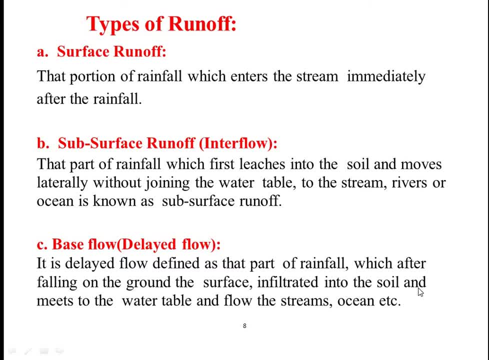 the ground surface, infiltrate into the soil and meets to the water table and flow to the stream, oceans, etc. The movement of water in this type of runoff is very slow. That is why it is also referred as delayed runoff. Sometimes base flow is also known as groundwater flow Coming to the 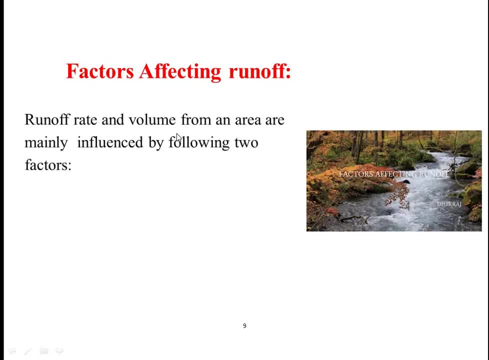 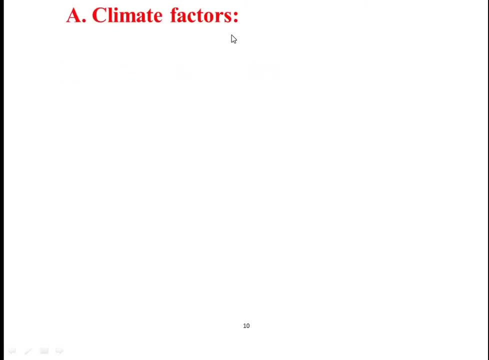 factors of effect Effecting runoff. Runoff rate and volume from an area are mainly influenced by following two factors: First factor is the climatic factor and second factor is the physiographical or topographical factor. Coming to the climatic factors, First one is the types of precipitation. It has great effect. 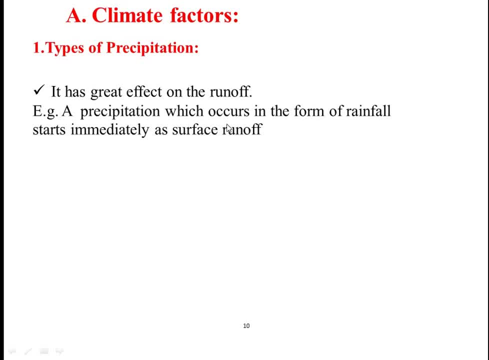 on the runoff Example, a precipitation which occurs in the form of rainfall starts immediately at surface runoff, Depending upon rainfall intensity, while precipitation in the form of snow does not result in surface runoff. Then second one is the rainfall intensity. If the rainfall intensity is greater than the 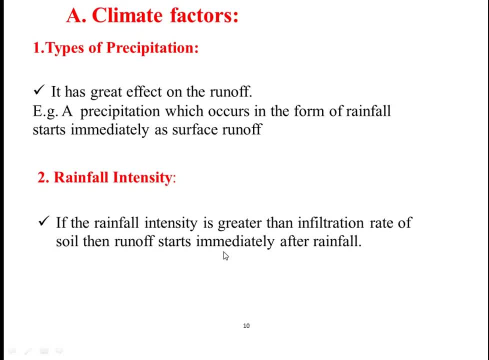 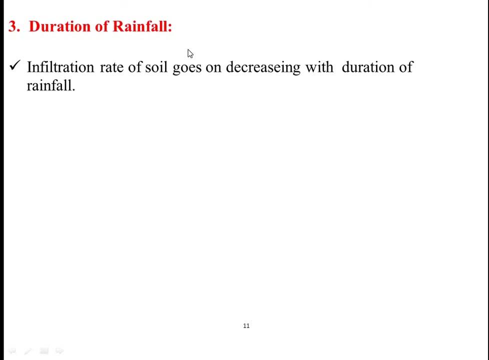 infiltration rate of soil, then runoff starts immediately after rainfall, While in case of low rainfall intensity, runoff starts later or will be generated. High intensities of rainfall yield higher runoff Duration of rainfall. It is directly related to volume of the runoff, because the infiltration rate of soil goes on. 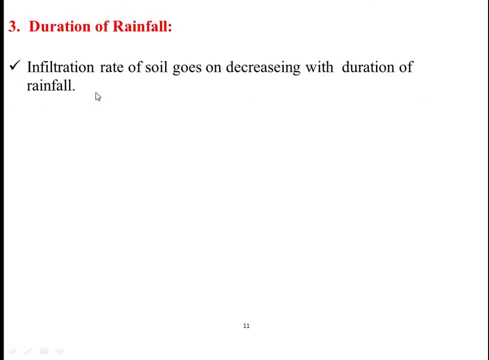 decreasing with duration of rainfall. Therefore, medium intensity rainfall even results in considerable amount of runoff if duration is longer. Even a mild intensity rainfall lasting for longer duration may increase yield a considerable runoff. Then rainfall distribution. Runoff from a watershed depends very much on the distribution of rainfall, The ratio of maximum rainfall at a point to a mean. 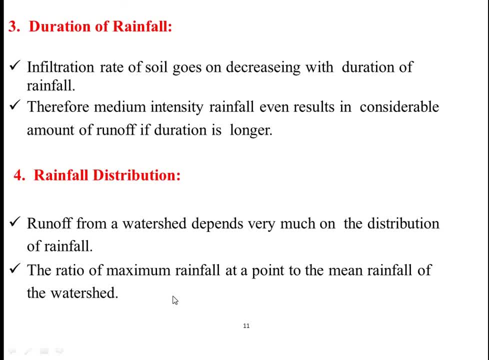 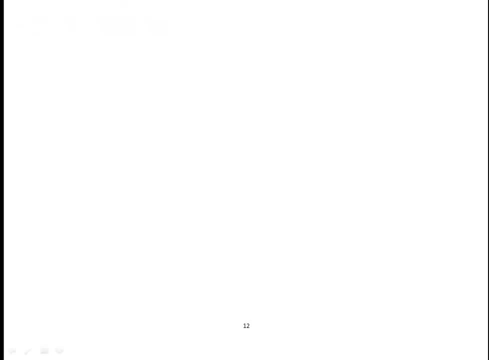 rainfall of watershed, termed as distribution coefficient. The greater the value of distribution coefficient, greater will be the peak runoff. Peak runoff would be resulted from the storm flow falling on the lower part of watershed. Then, direction of prevailing wind. If the direction of prevailing wind is same as drainage system, it results in peak flow, A storm moving in the. 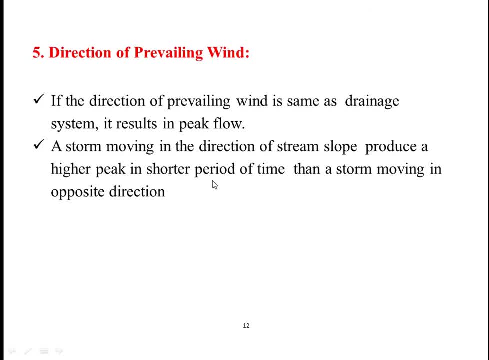 direction of stream slope produce a higher peak in shorter period of time than a storm moving in opposite direction. Then other climate factors. Other climate factors such as temperature, windoll, Wind velocity, relative humidity, annual rainfall etc. affect the water losses from watershed area. 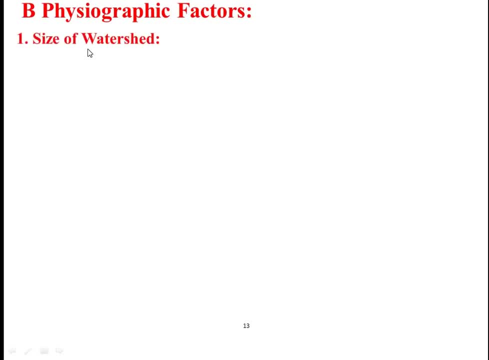 Coming to the physiographic or topographic factors. First one is the size of watershed. A large watershed takes longer time for dragging the runoff to the outlet. As a result, peak runoff is being smaller. The shape of watershed Runoff is greatly affected by shape of watershed. 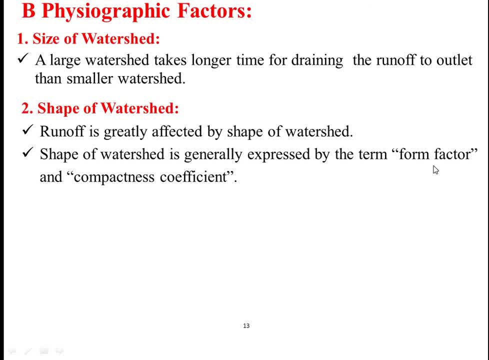 Shape of watershed is generally expressed by the term form factor and compactness coefficient. Form factor is defined as ratio of average width to axial length of watershed, And compactness coefficient is defined as ratio of perimeter of watershed to circumference of circle whose area is equal to area of watershed. 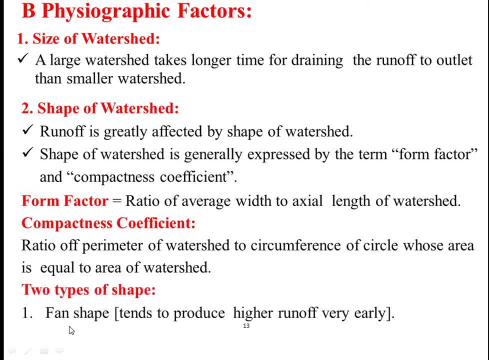 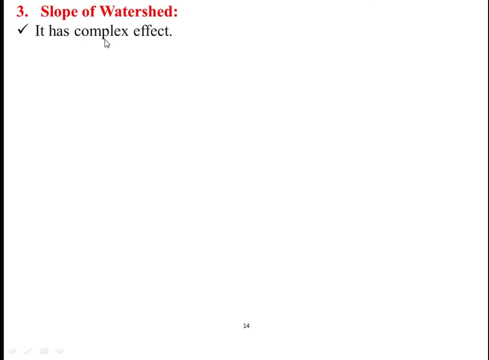 Then there are two types of shape. First one is the fan shape That tends to produce higher runoff very early, And second type one is the fern shape That tends to produce less runoff Slope of watershed. It has complex effect. It controls the time of overland flow and time of concentration of rainfall. 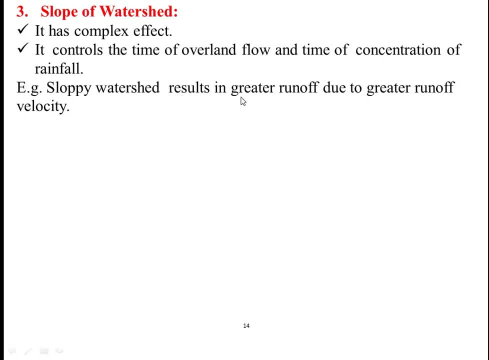 For example, in case of slopey watershed, the time to reach the flow at outlet is less Because of water, Because of greater runoff, Because of velocity. This results into formation of peak runoff very soon. Then orientation of watershed: This affects the evaporation and transpiration losses from the area. 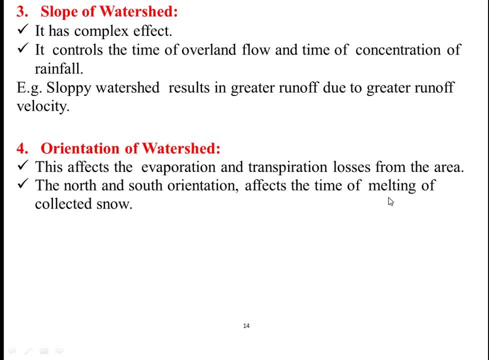 The north and south orientation watershed affects the time of melting of snow. The windward side of the watershed receives high intensity of rainfall, resulting into more runoff, While part of watershed lying toward leeward side has reverse trend. Then land use. Land use and land management practices have great effect on the runoff yield. 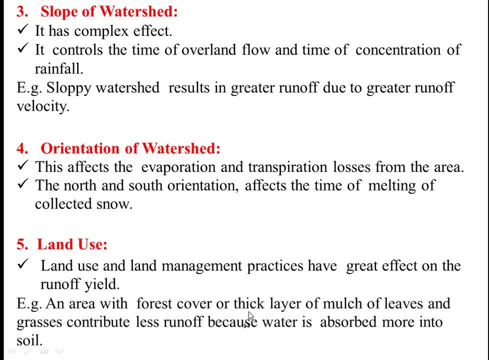 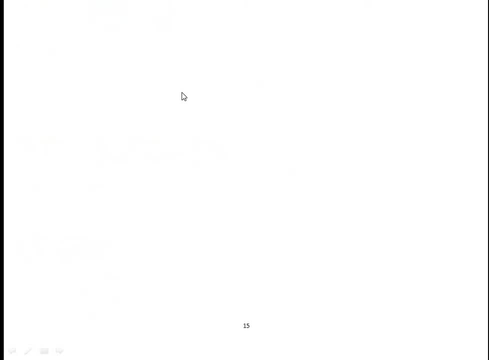 For example, an area which under forest cover or with thick cover of mulch of lewds and grasses, Then the formation of surface runoff is very less, While in barren field generation of runoff is more. Soil moisture Magnitude of runoff yield depends upon the initial moisture present in soil at the time of runoff. 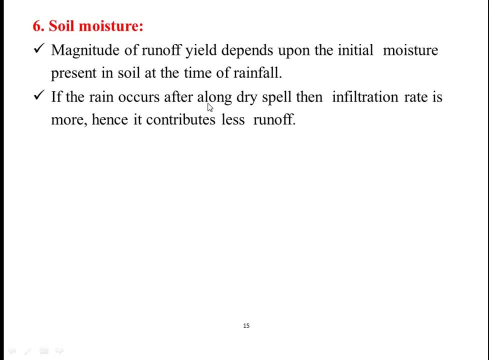 Soil moisture. If rainfall occurs over the soil which has more moisture, the infiltration rate becomes very less, which results in more runoff. When the soil is dry, causing to absorb huge amount of rainwater, results in less runoff. Then soil type: Infiltrate rate vary with type of soil.